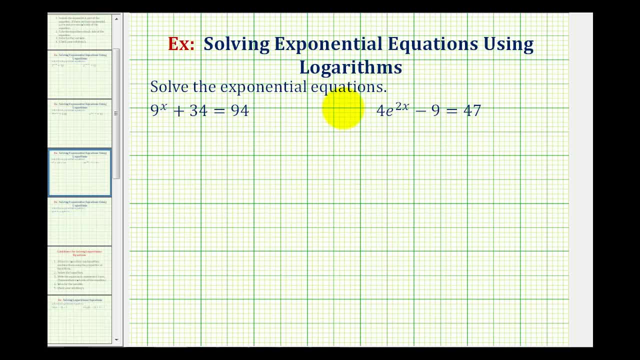 We want to solve the given exponential equations using logarithms. If an exponential equation has only one exponential part, like these two examples, we want to isolate the exponential part and then take the log of both sides of the equation to solve for the variable. 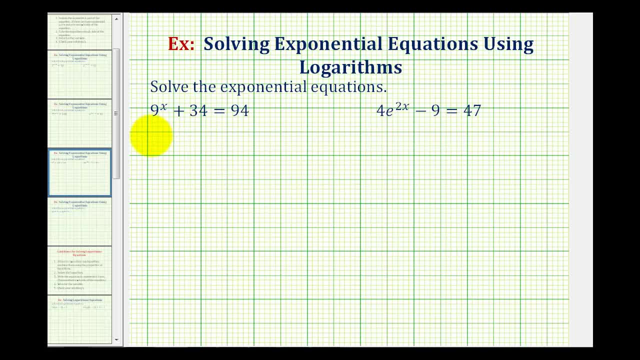 So, looking at our first equation, we have nine raised to the power of x plus thirty-four equals ninety-four. Again, our first step is to isolate the exponential part, or isolate nine raised to the power of x. So we want to undo this addition, so we'll subtract. 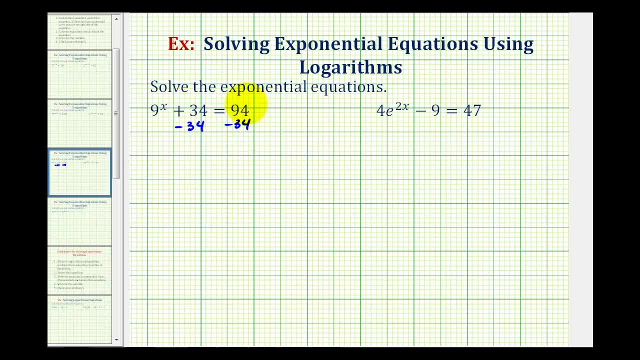 thirty-four. on both sides of the equation This would be zero. so now we have nine. raised to the power of x equals sixty. Now that we have the exponential part isolated, we're going to take the common log or natural log of both sides of the equation And we use common log or natural log. 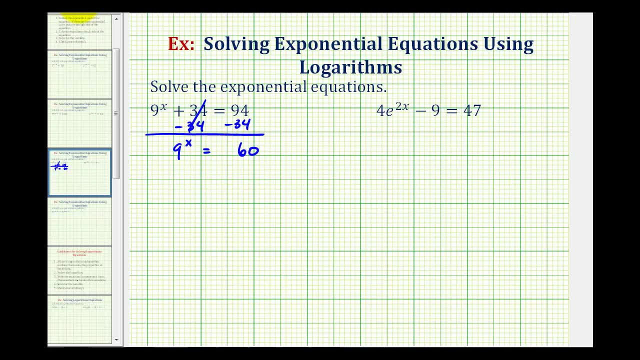 because we'll have to use the calculator to solve this. for x, Let's go ahead and take the natural log of both sides of the equation And now, on the left side of the equation, we can apply the power property of logarithms and move this exponent to the front. So now we have x times natural log nine. 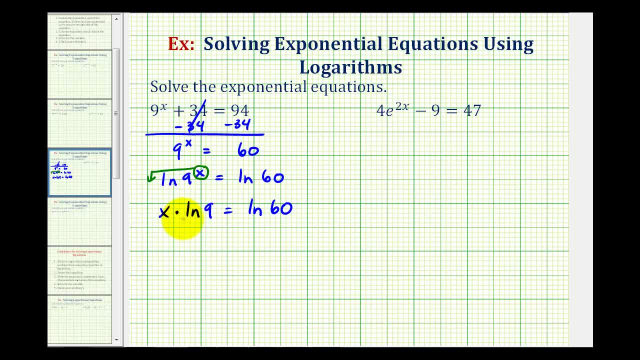 equals natural log sixty. And now to solve for x. we can undo this multiplication by dividing both sides by natural log nine. On the left side this simplifies to one. So we have x. equals this quotient here, which we'll have to get a decimal approximation for on the calculator. 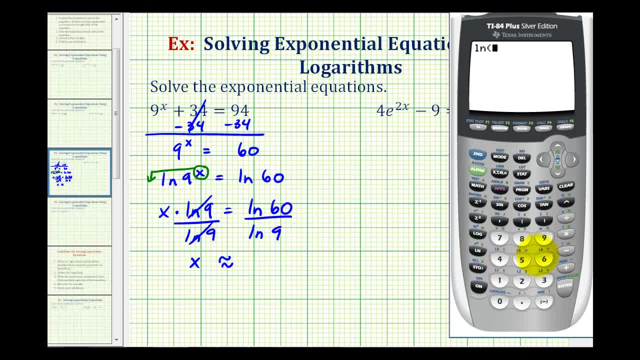 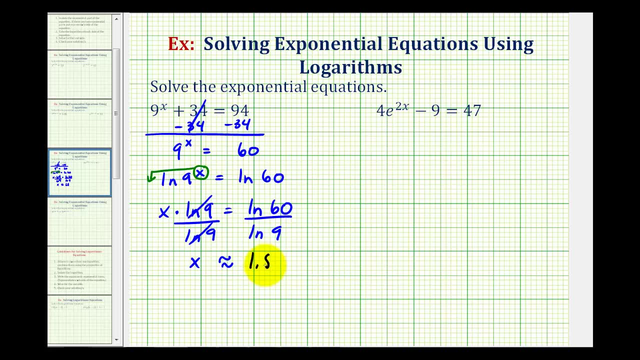 So we'll have natural log sixty divided by natural log nine, The standard to round to four decimal places. so x is approximately one point, eight, six, three, four. So if we sub this back into the original equation, this means that nine raised to the power of one point. 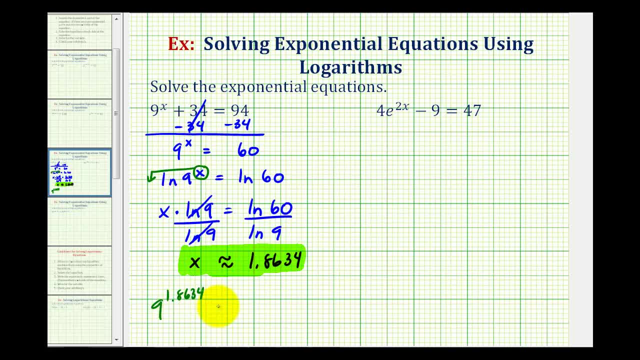 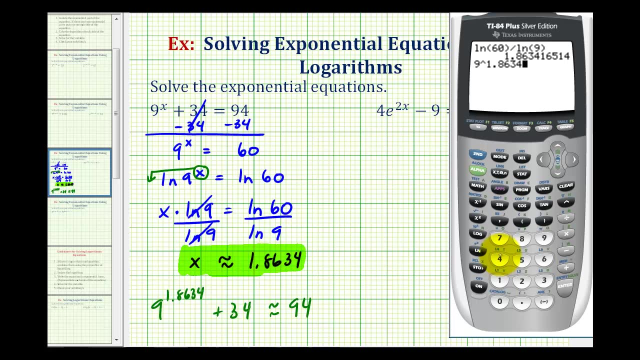 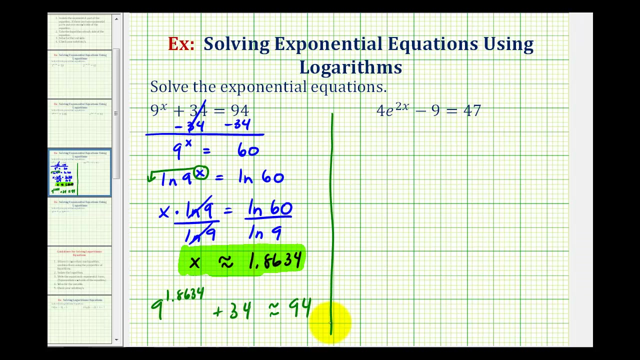 eight, six, three, four plus thirty-four should equal or be approximately ninety-four. Let's go ahead and check this And, because we did round down, the value is slightly less than ninety-four, but this does verify our answer. Looking at our second example, we want to isolate e raised to the power of two x. 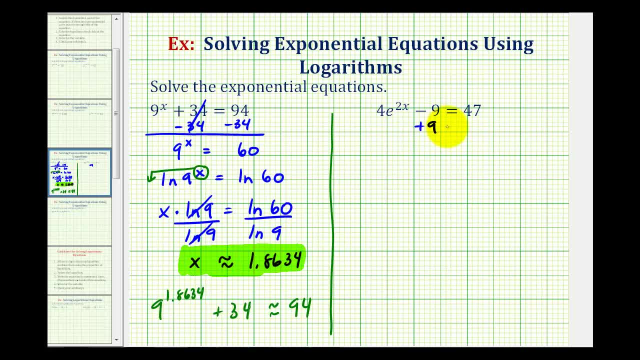 So for the first step we'll undo this subtraction by adding nine to both sides. So we have four times e raised to the power of two. x equals this is going to be fifty-six. And we also want to undo this multiplication here between d four. 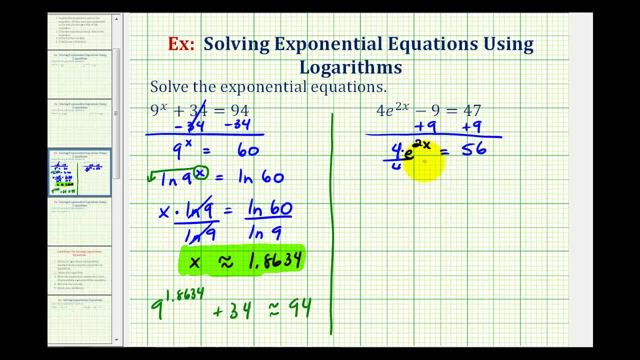 and e raised to the power of two x. So now we'll divide both sides by four. This simplifies to one. So we have e raised to the power of two, x equals fourteen. And now we'll take the log of both sides. And because we have base e here, 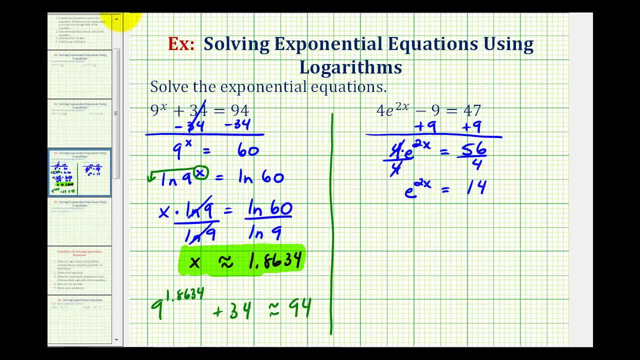 it'll be much easier if we take the natural log of both sides. So we'll have the natural log of e to the power of two. x equals natural log fourteen, And now we'll apply the power property of logarithms here, so we can move this. 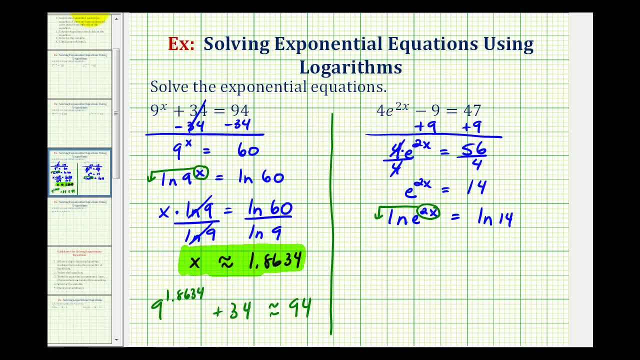 exponent of two x to the front. So this is now going to be two x times natural log. e equals natural log fourteen. Natural log e is actually equal to one. Remember, natural log is base e and e to the first power is equal to e. 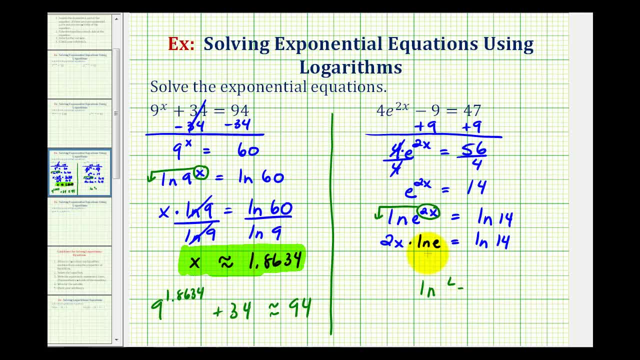 verifying that natural log e is equal to one. So we could just drop this natural log e. but just in case we didn't recognize this, we can now solve for x by dividing both sides by two. natural log e. Two over two simplifies to one. 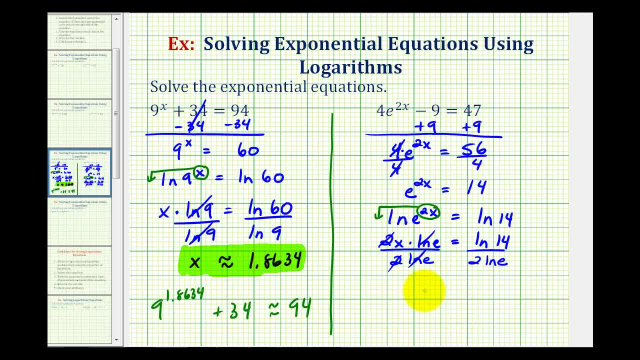 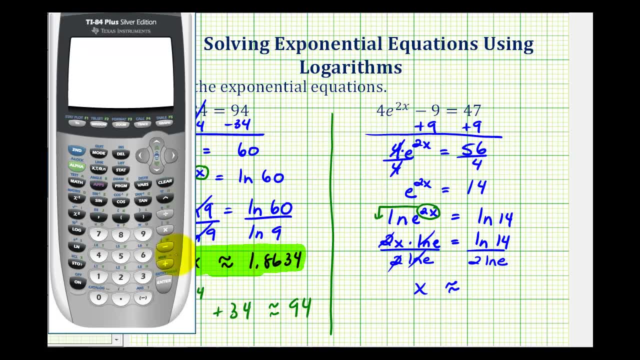 Natural log e over. natural log e simplifies to one. So x is equal to this quotient here, which we'll use a calculator to get a decimal approximation for. So our numerator is natural log fourteen and we'll divide this by two or two natural log e.